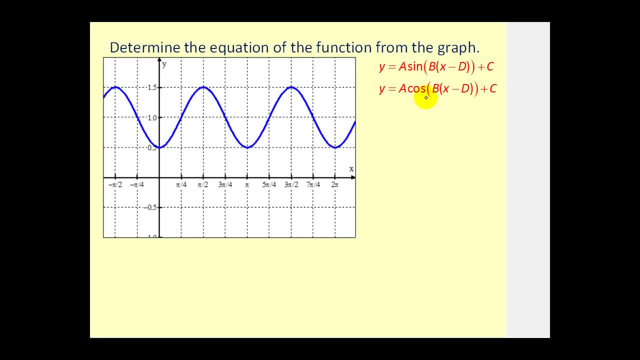 So, really, we have a choice on which of these equations we want to use, And the way we're going to do this is: first, we're going to pick a piece of the graph and we're going to highlight one period of it. So for this graph, I'm going to isolate this piece of the graph and you can see right away. 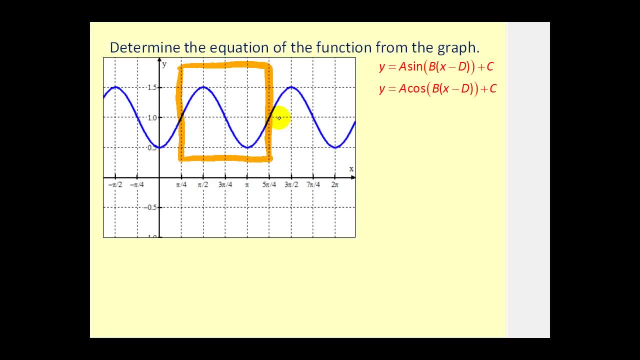 it resembles the graph, So we're going to use this form to find the equation of this graph. The next thing I recommend is drawing a horizontal line through the center of the graph like this, And what this does is make finding the amplitude easier. 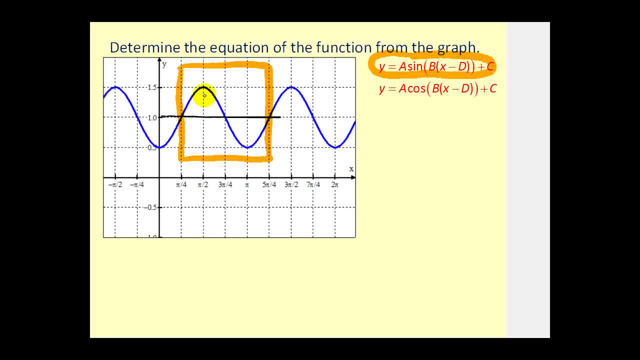 And we can see if this is the center line. this is the maximum. this distance is 1 half. Therefore, our amplitude is equal to 1 half, and so we know that A is equal to 1 half. The next thing that it shows us is that, typically, the sine function hugs the X axis. 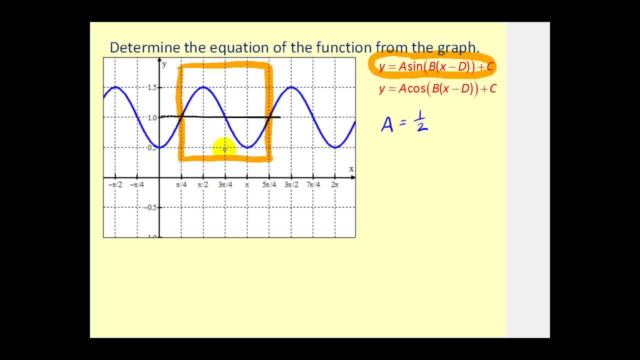 or the X axis is the center of the graph And we can see now it's been shifted up 1, so now we know that C is equal to 1.. So now what we have to do is find the period and the phase shift or horizontal shift. 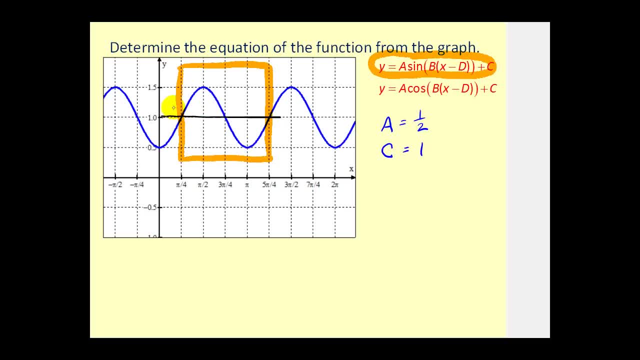 What we can also tell that from the basic sine function, this graph has been shifted pi over four units to the right. So that tells us that D is going to be pi over 4.. pi over four. And lastly, we need to find the value of b. 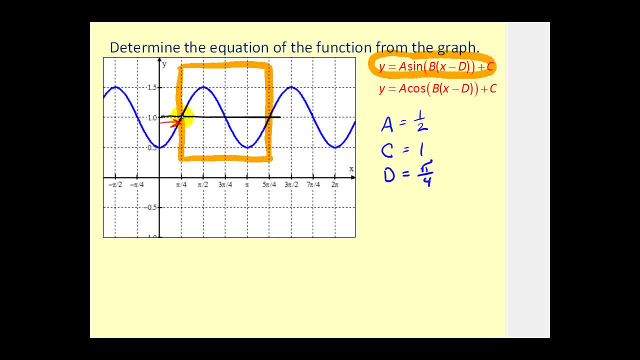 and we can figure that out from the period. Notice that from pi over four to five pi over four, we have one complete cycle of this sine function. So five pi over four minus one pi over four is four, pi over four or pi radians. 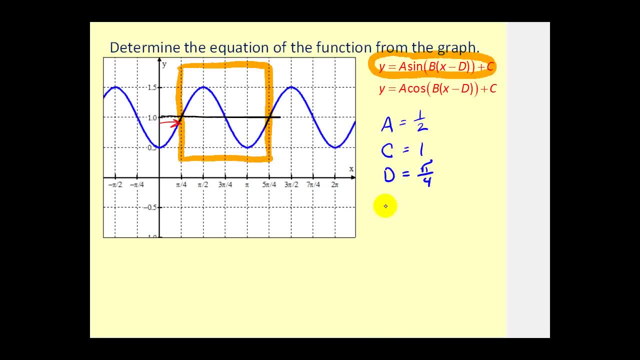 So the period is pi radians. Remember, the period is equal to two pi divided by b, and again we're saying that's equal to pi radians. So we can do cross products. here We have b. pi is equal to two pi dividing by pi. 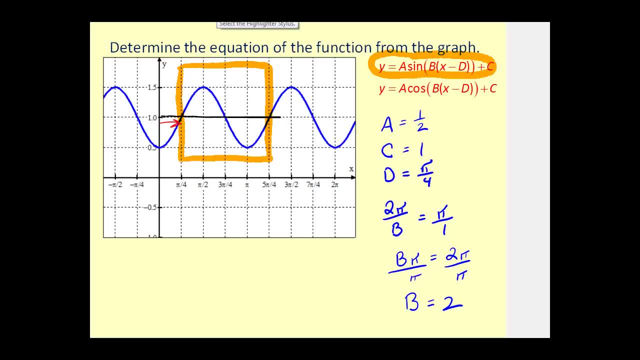 We have b equal to two. This is all the information we need. We have a, b, c and d, So let's write our equation: Y equals one half sine of two pi over four of the quantity b times the quantity x minus d. 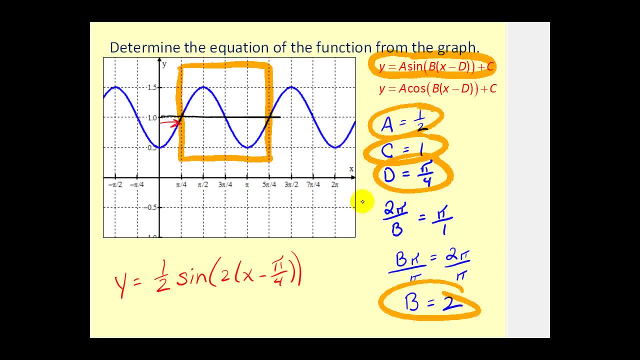 D is pi over four plus c, and our c value is one. Okay, so let's check this out: Our amplitude is one, half, Our period two. pi divided by two is pi radians, The phase shift, remember if it's minus pi over four. 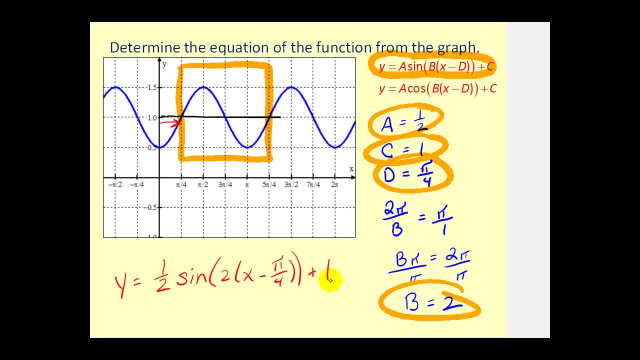 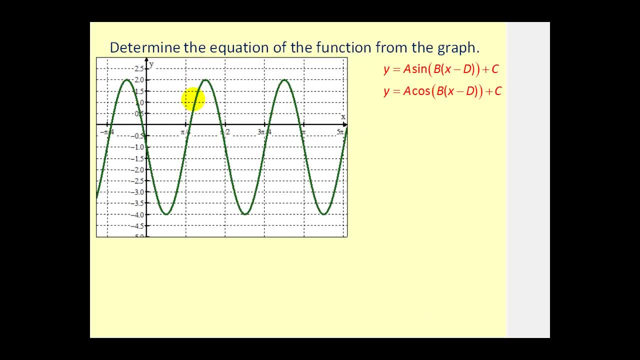 that means right pi over four and then up one. So there we go, Let's try another. First, let's take a look at the graph and determine which piece of the graph we want to focus on. We want to highlight one period of what looks like. 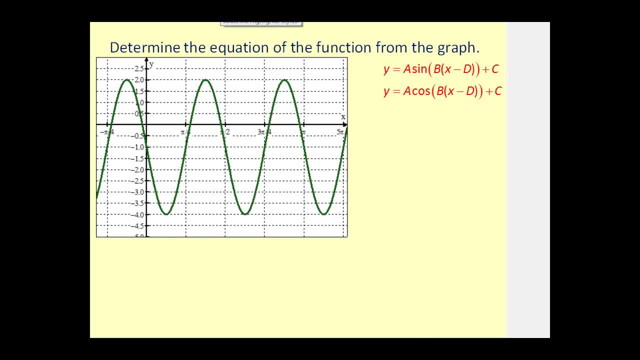 either the graph of sine or cosine, and this is why the equation that we find will not be unique. So when I look at this, I see the graph of a sine function starting at pi over four, going up down and then back up. 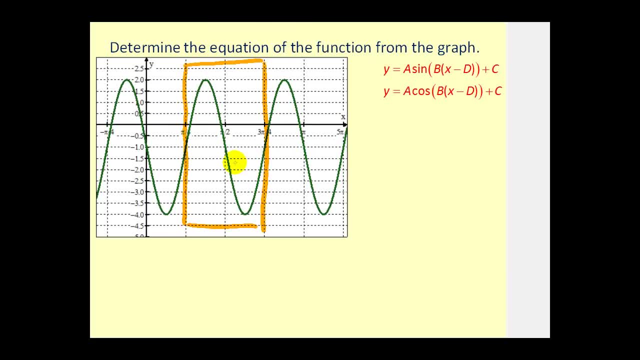 So we'll use this piece to find the equation of this function and again you can see we're going to use the sine function. Next, we'll draw a line through the center. Looks like it's going to be at negative one. 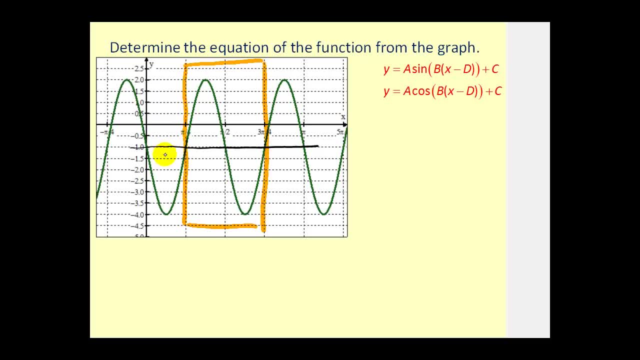 So, by the way, when we draw the center line through, y equals negative one. we know that our vertical shift c will be negative one. Next, the amplitude from negative one to positive two would be three units, so a is equal to three. 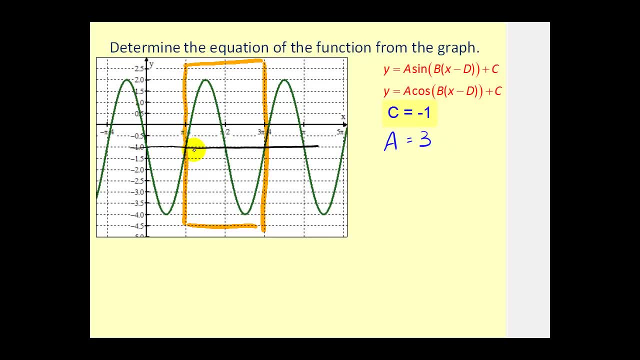 The phase shift again is right: pi over four units, so d is equal to pi over four. And now we have to determine the period so we can find the value of b. Remember two pi divided by b is equal to our period. 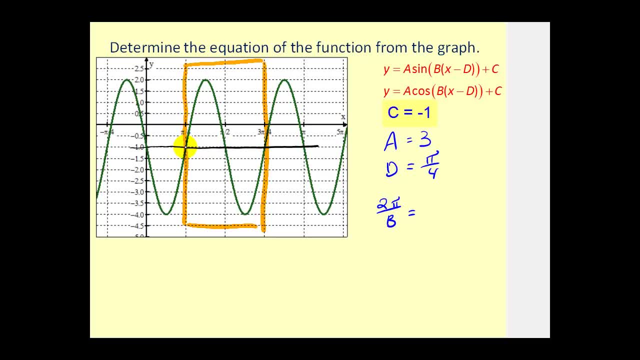 so we have three pi over four, minus one pi over four would be two pi over four or pi over two, And again we'll perform cross products here. B times pi must equal four pi dividing both sides by pi. So we have b equals four. 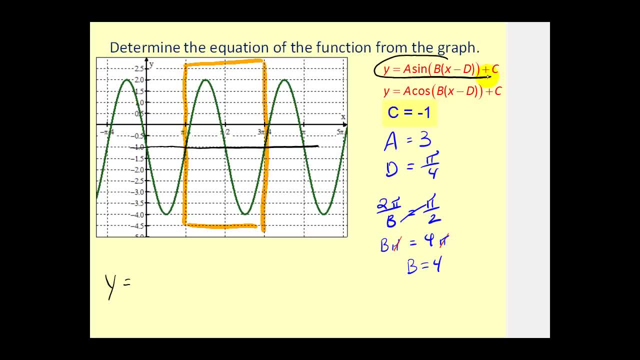 And that's all we need. Again, we're focusing on the sine function. So we have: y equals three sine of the quantity b, which is four X minus d, so x minus pi over four, And the shift was down one. so c equals negative one. 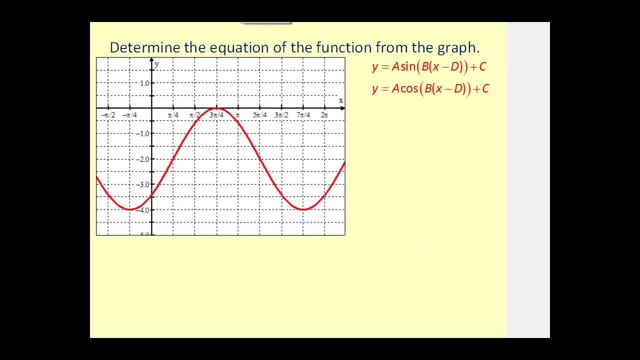 Okay, let's take a look at one more. Let's identify the piece we want to focus on, And for this one I'm going to focus on cosine. So we'll start here at this point and end at this point, Because from there on it starts to repeat. 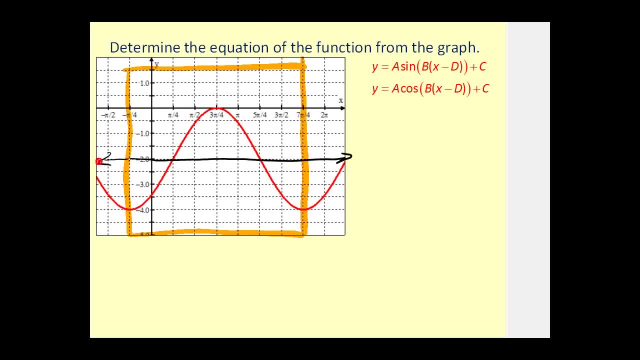 Draw a line through the center Looks like it's at. y equals negative two. So right away we know that c is equal to negative two. Next, we can see the distance from our center to a maximum is two units. We're looking at this graph. 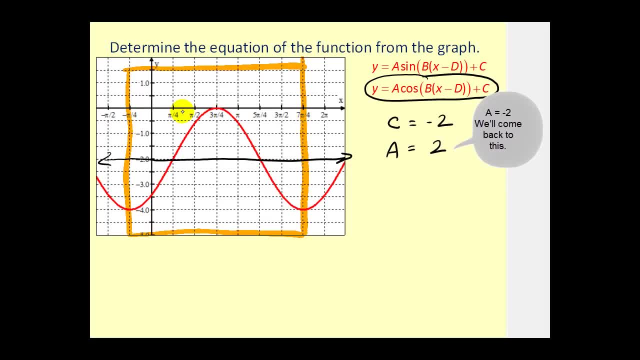 on the interval from negative pi over four to seven pi over four. That horizontal distance is two pi, So our period is two pi, which makes b equal to one. And lastly, we need to find d, The horizontal shift or phase shift. 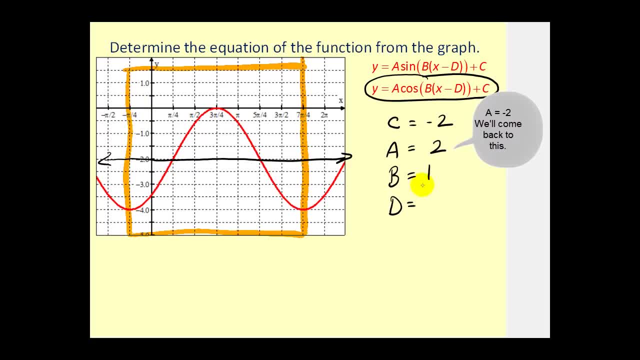 is left pi over four units. So d is actually negative pi over four. Now there's one other thing. Typically, when we graph the cosine function on the interval from zero to two pi, it looks something like this, And notice that we usually start at a maximum. 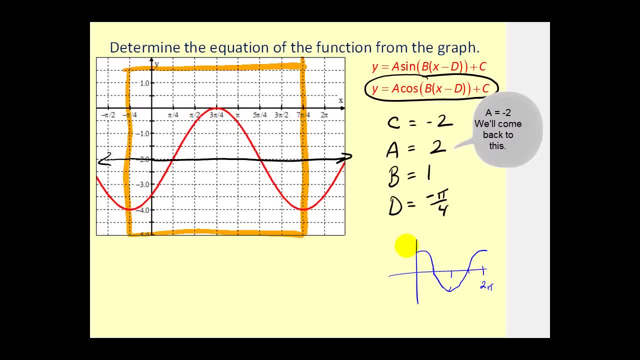 but now we're starting at a minimum. So what happened was the cosine function was reflected across the x-axis before it was shifted down two units. The result is: a is equal to negative two. So we have all the information we need now We have: y equals negative two. 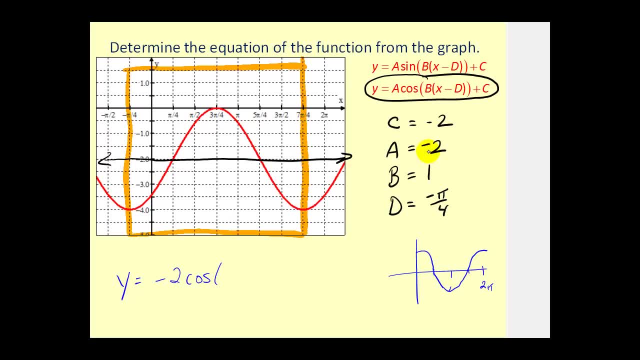 cosine. our b value is one, so we'll leave that off. And then we have x minus d. well, minus a negative pi over four is plus pi over four and then minus two. Now, on this problem, I did pick a more challenging piece. 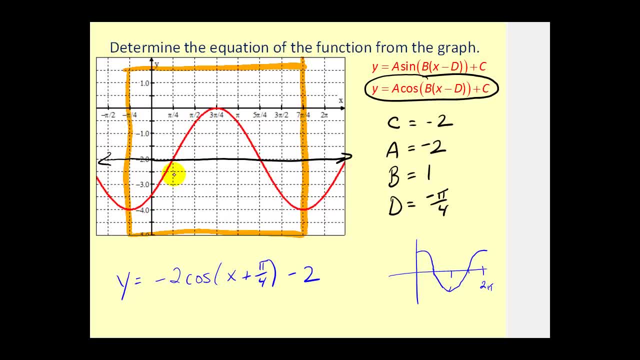 of the graph to find the equation to this time. Remember, these equations are not unique, so we could have chosen a different piece of this graph to find an equivalent equation in a different form. Okay, I hope you found this video helpful. Thank you. Thank you.